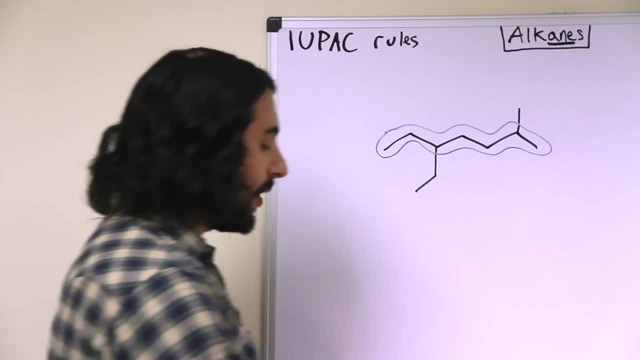 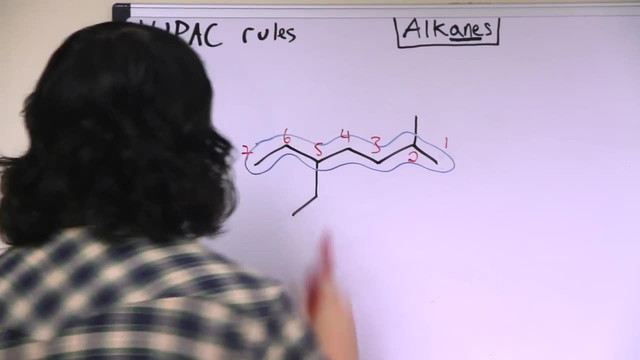 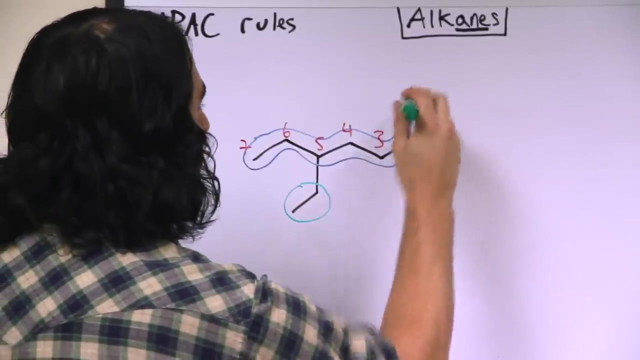 from the left. it would occur on the third. so we're going to number this right to left and we are going to see that there are therefore two alkyl substituents. we have a two carbon substituent here and a one carbon substituent here. so that means 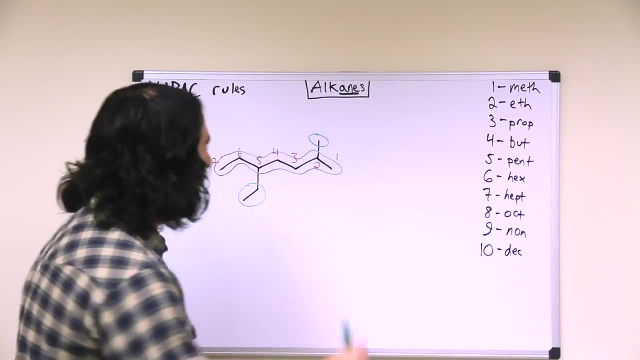 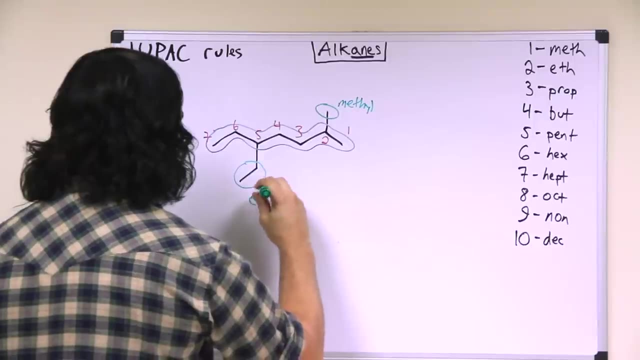 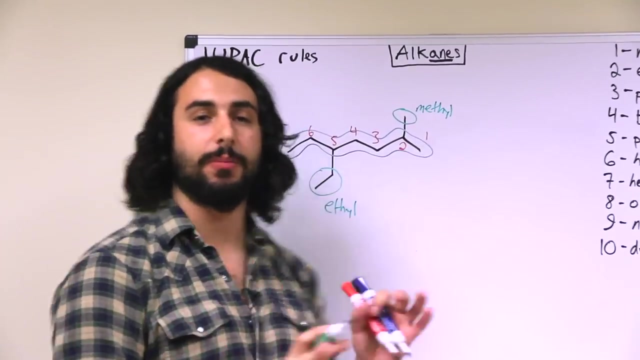 that this molecule overall is a heptane and there is a methyl substituent and this two- carbon substituent- is an ethyl substituent. so we know that this is a heptane. but now, separately from the algorithm that we use to number the, 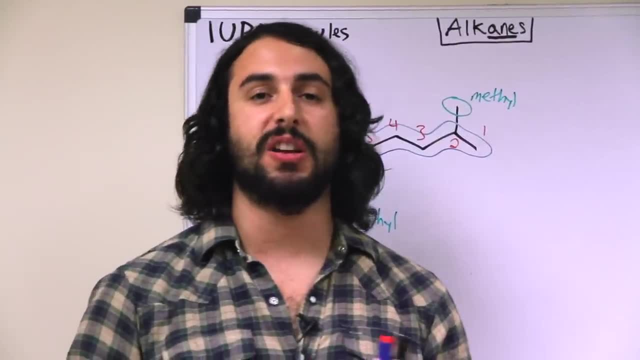 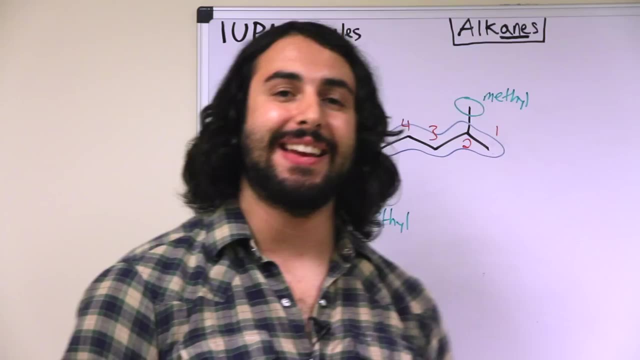 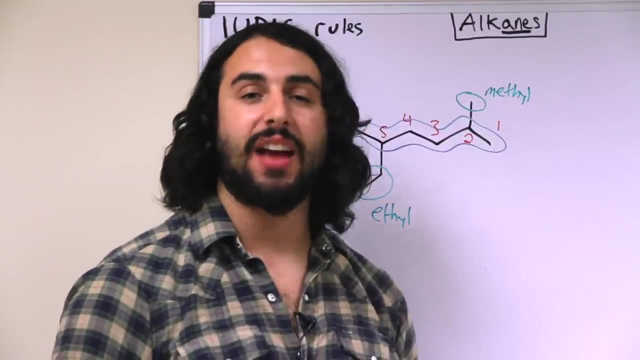 molecule. a different algorithm is going to be used to figure out in what order we name all the parts of the molecule, so we are going to have to list these in alphabetical order. so ethyl starts with E, methyl starts with M and for that. 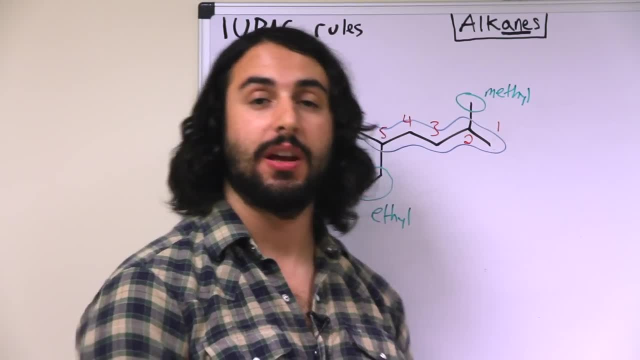 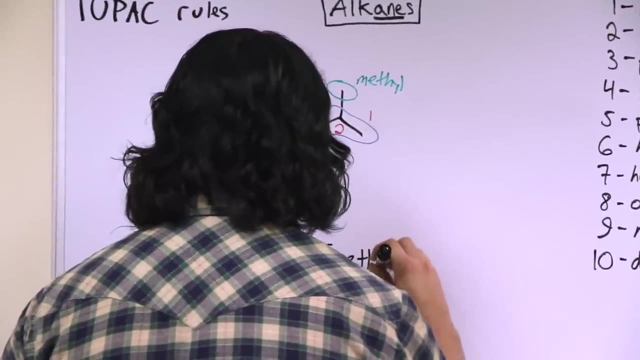 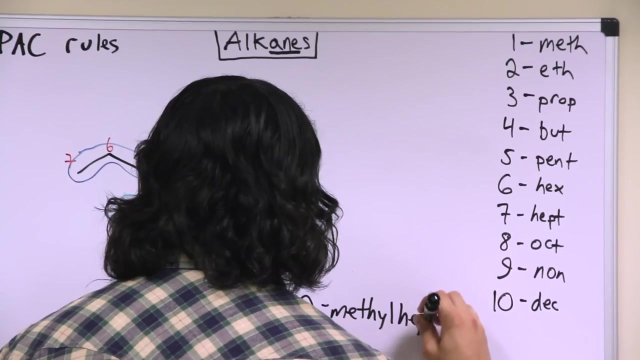 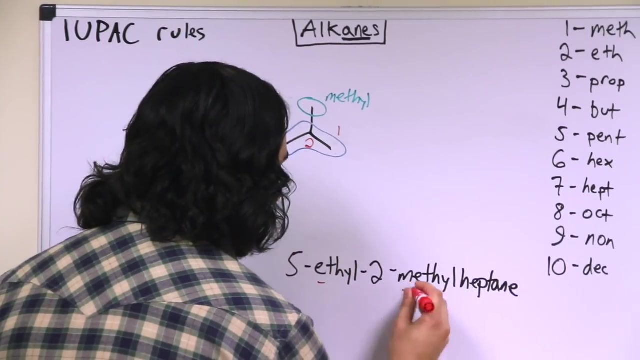 reason alone, we are going to list the ethyl group first, on the carbon that it occurs. so that is five ethyl, two methyl heptane. so once again, this is a completely arbitrary rule, but if we all follow it we will be able to come up with the same name for the molecule E. 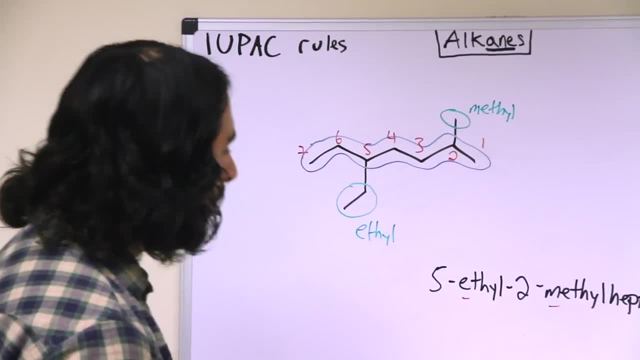 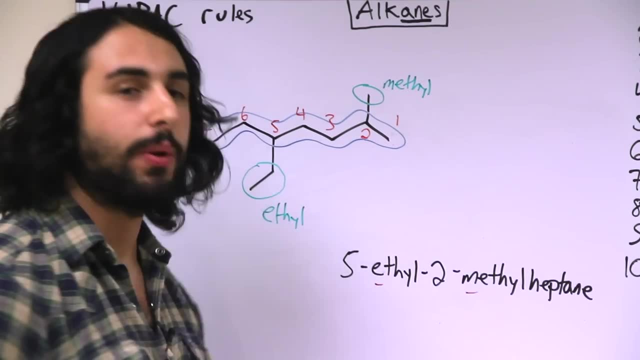 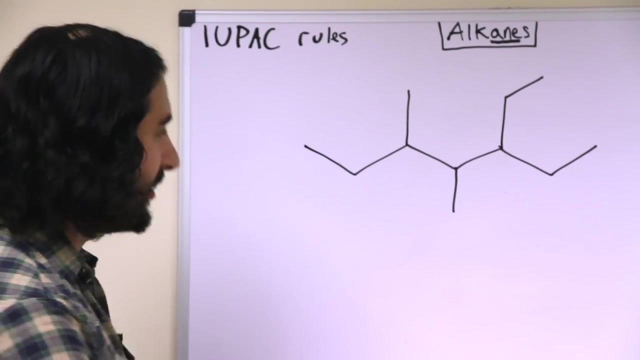 before M. ethyl before methyl. just as a point of convention, in between words and numbers we will have a hyphen, and later we will see that in between numbers there is a comma. let's look at a slightly trickier example. once again, the first thing we're 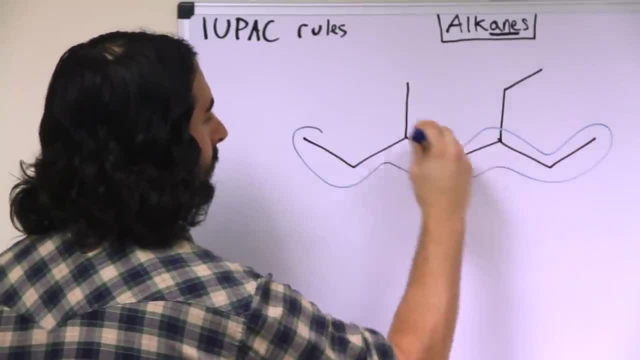 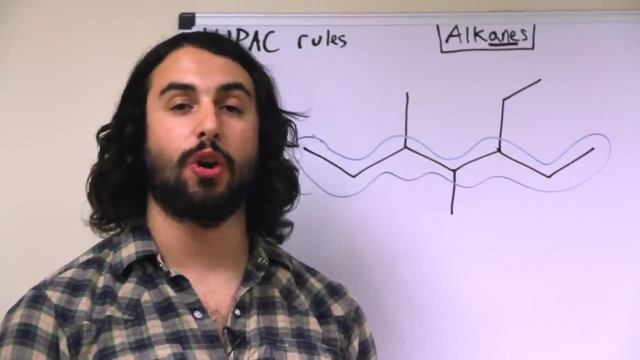 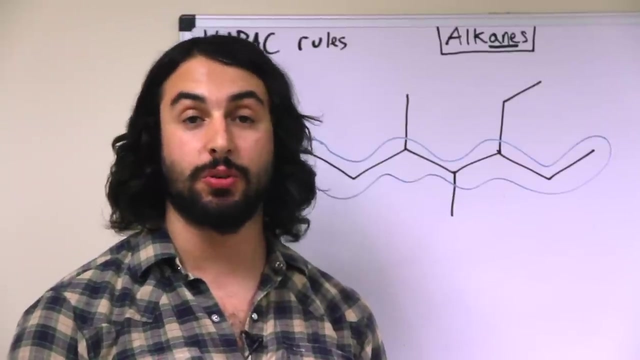 going to do is identify the longest carbon chain. now, in the case that we have a substituent occurring at the same position, regardless of whether we begin numbering from the left or the right, we are going to give priority to the substituent that occurs soonest alphabetically. so in this case, because 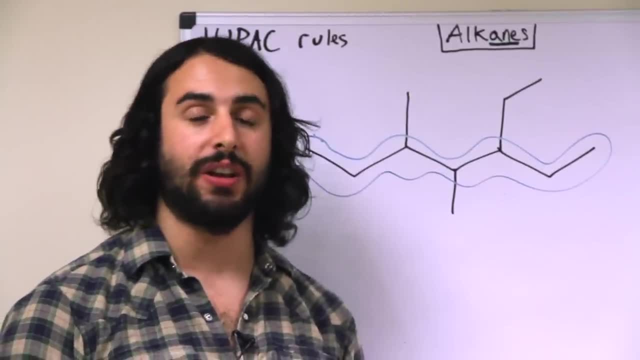 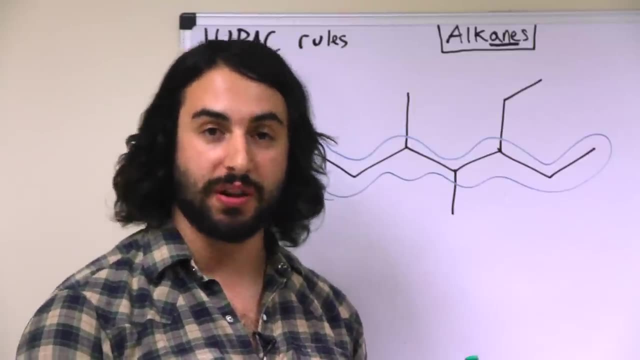 they are both alkyl substituents. they have the same priority. later we will see other types of substituents that take priority over alkyl, but in this case we're just going to go with alphabeticity. so we have a methyl and we have an ethyl. 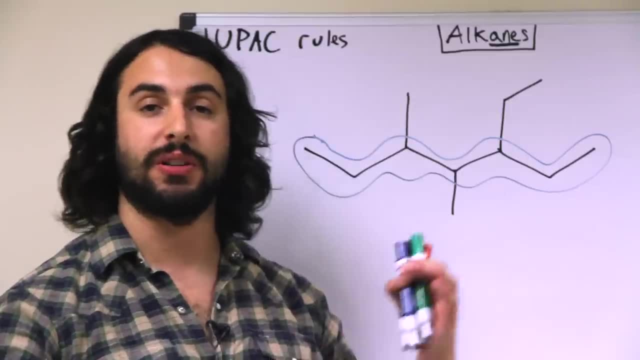 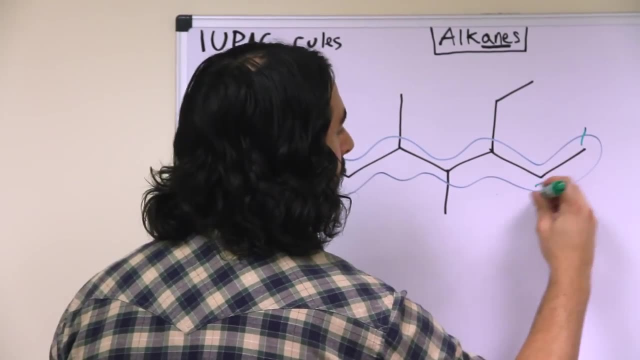 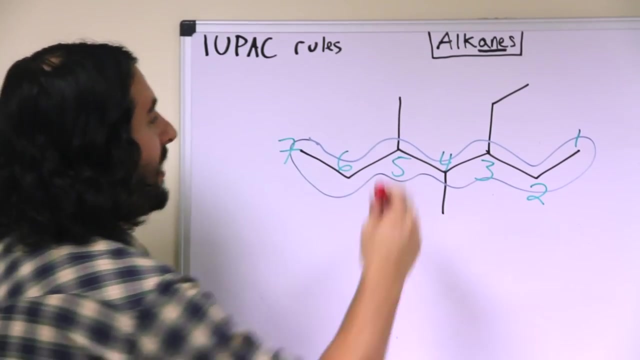 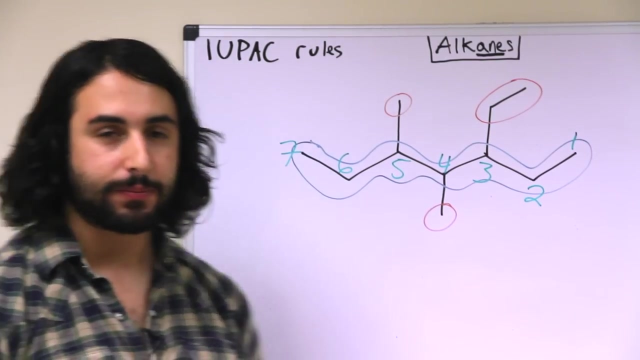 occurring on carbon 3, regardless of whether we start from the left to the right, but ethyl before methyl, alphabetically, so we will number right to left. so now we identify that we have a methyl group on carbon 5, a methyl group on carbon 4, and an ethyl group on carbon 3.. now, if it is the case that we 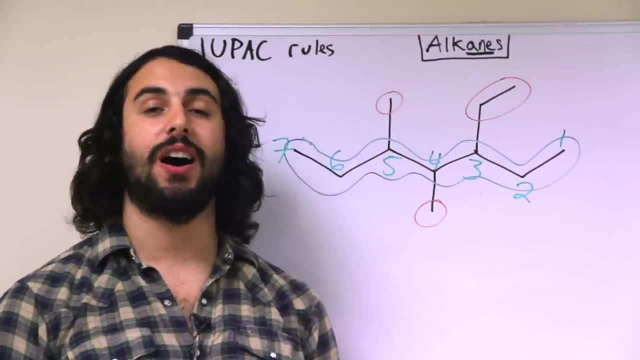 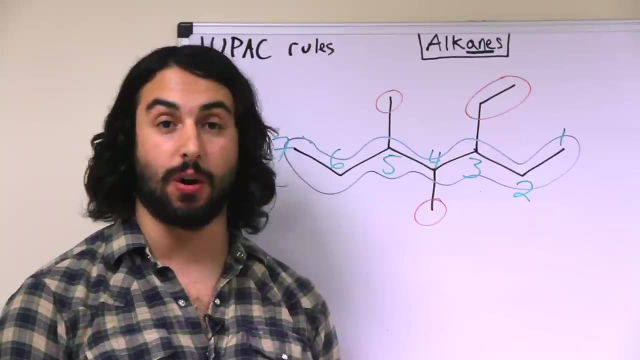 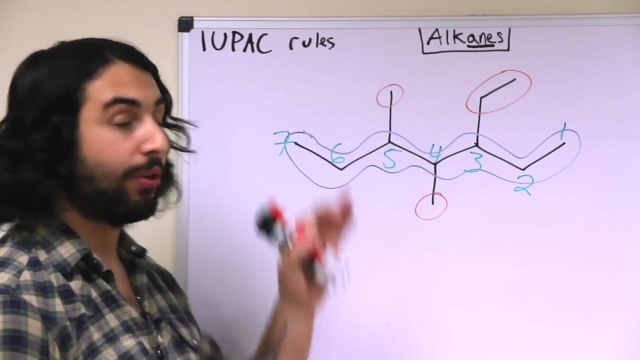 have multiple substituents of the same type on a given molecule, we're going to list them simultaneously with a prefix indicating how many of them there are. but that prefix will not be taken into account for alphabeticity. so ethyl still is before methyl, so we will write that first. so we have three. 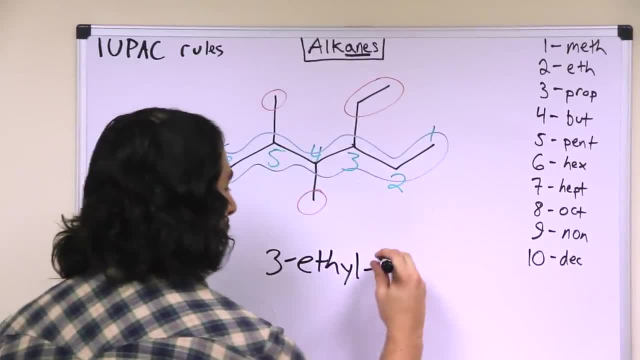 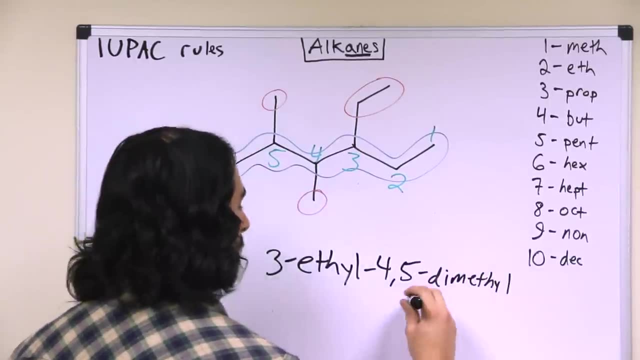 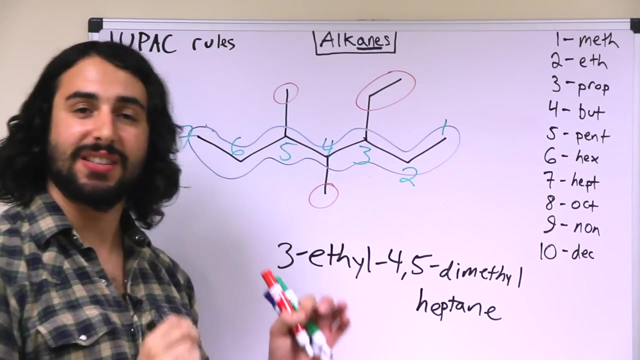 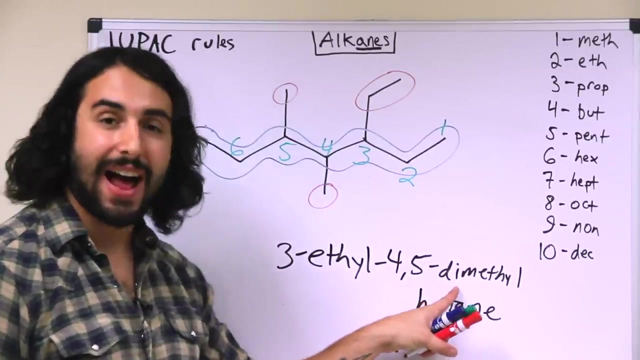 ethyl, and then we are going to say 4,5-dimethylheptane. so the point is that we have identified that there are two identical methyl groups, so we want to list them at the same time, but with the prefix di-, indicating that there are. 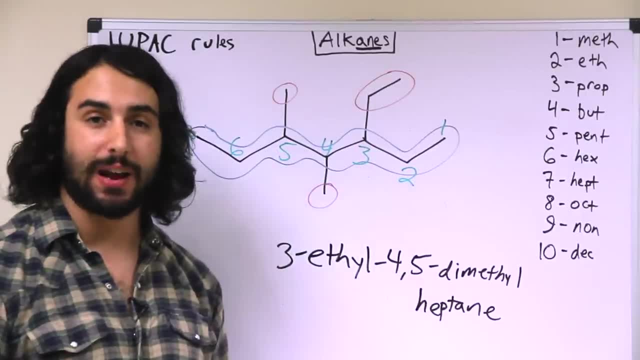 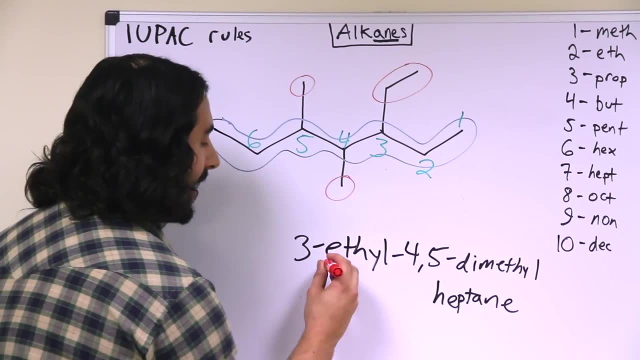 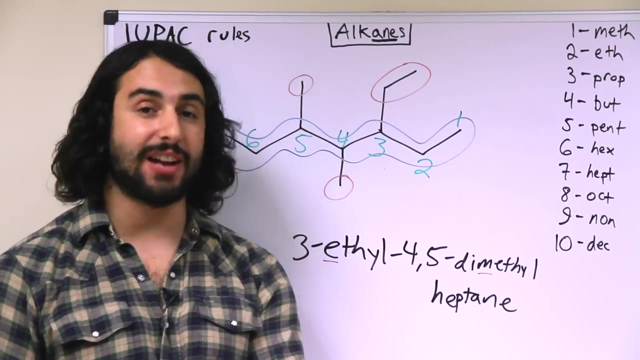 two of them and then the numbers four and five, separated by a comma, indicating that they occur on carbons four and five in the molecule. however, it remains the case that E before M, in other words these prefixes which would be di-, tri- or tetra-, are not taken into account for the 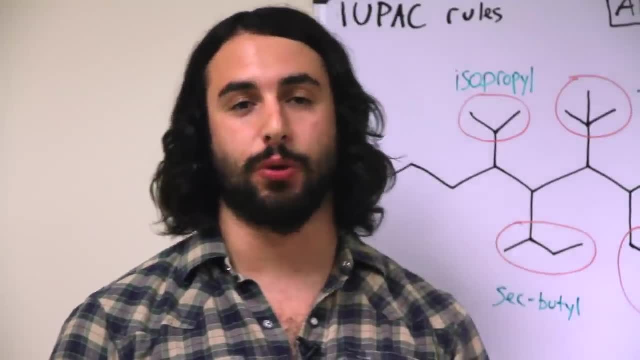 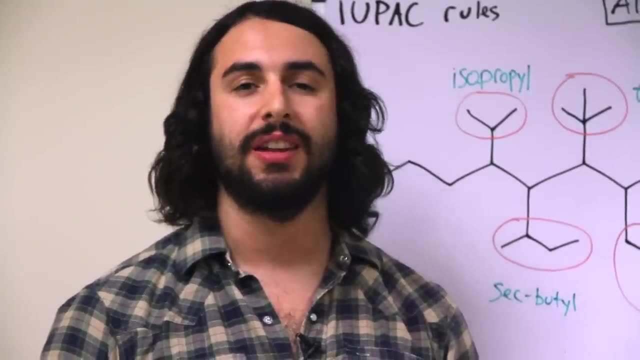 alphabeticity. okay, now let's take a look at a couple of groups that have names that are common names. they don't follow IUPAC rules, but we use them so frequently that we're going to need to know how to use them regardless. so don't pay attention to the main molecule. I just 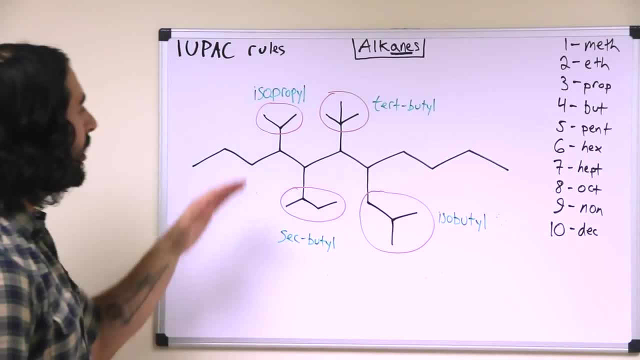 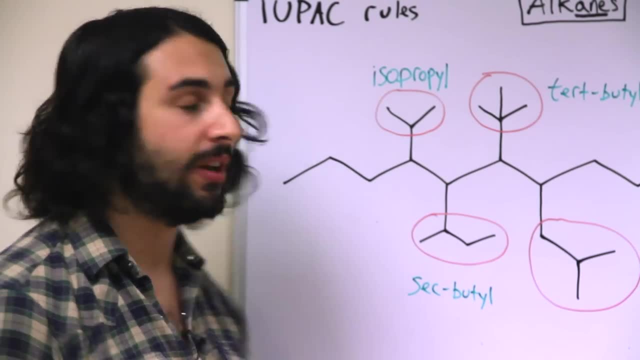 drew a molecule to show you these different kinds of substituents. this first one is an isopropyl group. so it's a propyl group because it is a three-carbon alkyl substituent and iso is regarding to the shape. basically, if